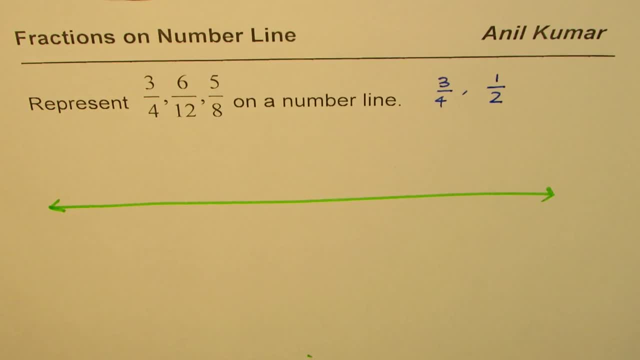 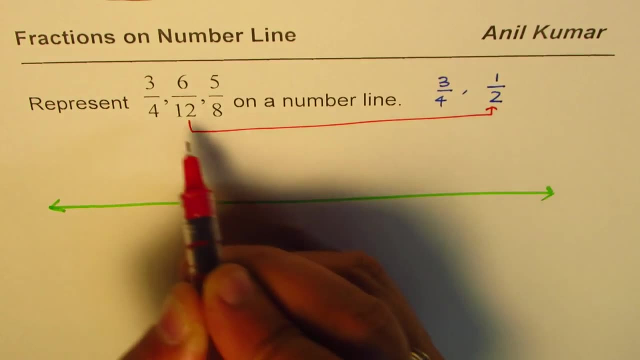 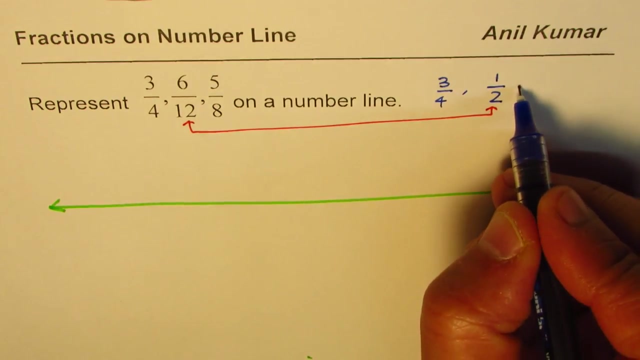 that. So 6 out of 12 can be written as half, dividing both by 2.. So this number here could be written as half, since we can divide both by 6 and then we get this number and then we have 5 out of 8.. So think like this: 5 out of 8 is like 4 plus 1. So slightly more than half. 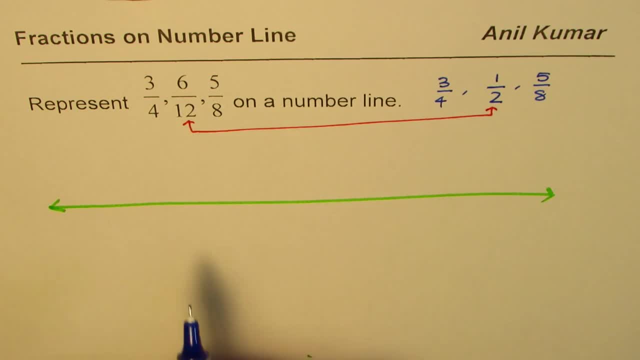 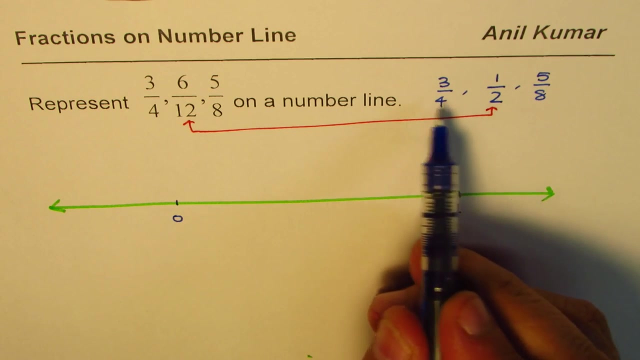 Do you see? Anyway, we'll draw that. Let's explore it more while plotting on a number line, And let us say that this is the 0 for us. Okay, and let's take a number 1 here somewhere and this is, let's say, number 1.. Now, all these 3. 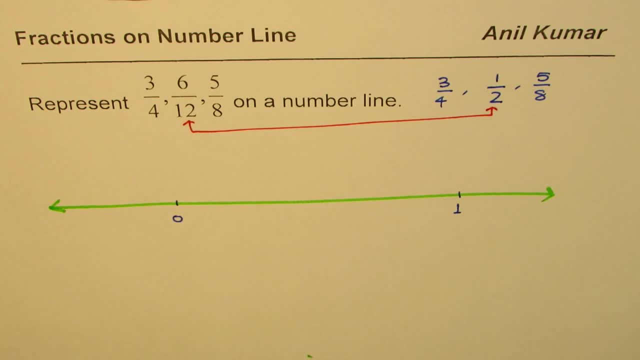 fractions which we are talking about are between 0 and 1.. So that is one thing. we know Now how to represent them on number line. Half is probably the easiest number. Just go to the center of this and let us say that this is: 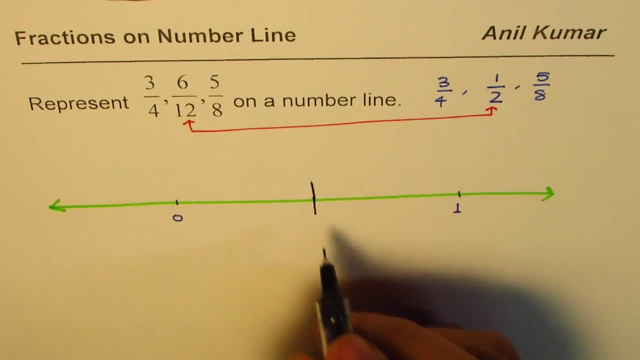 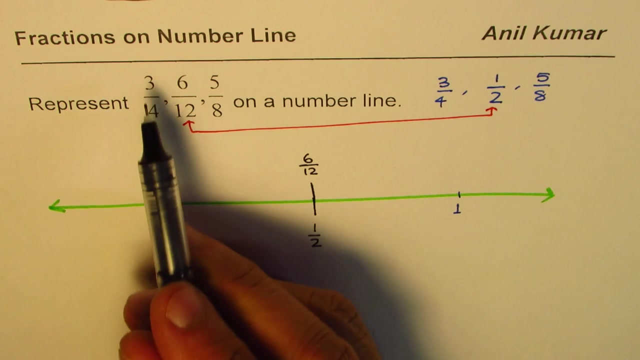 half for us, right? so let me draw a big line here. it's saying half and i'll write half here. so half or 6 by 12 is same thing, right? 6 by 12 is same as half. so we got the first fraction, which is half. now to get 3 over 4, we have to divide this number 1 into 4 equal parts. 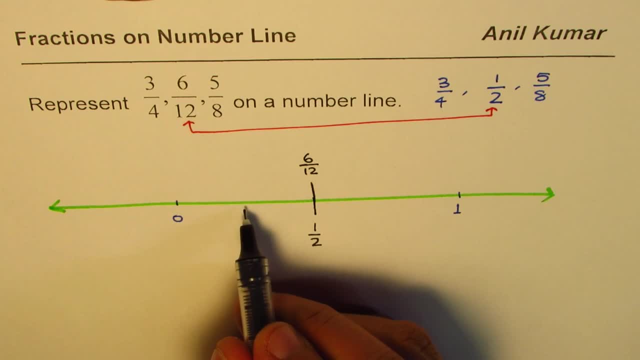 right now. 4 equal parts means half of half is one fourth. so so this is our. let us say, these are one fourths. now, right now, we know this is, uh, one fourth. right, let me write down: one fourth half could also be written as 2 out of 4. this could be written as 3 out of 4. in that case, that 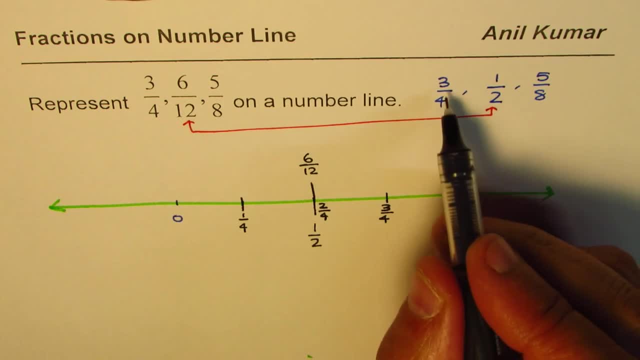 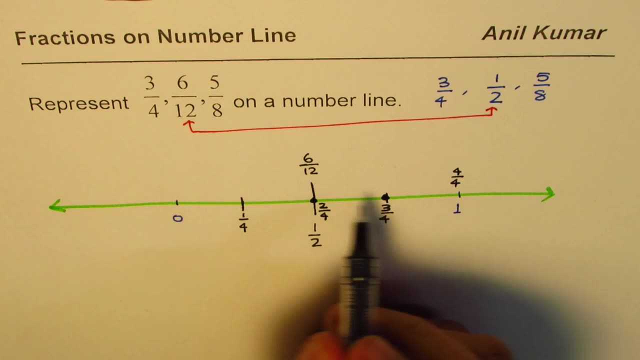 becomes what? 4 out of 4, right, since we need to represent 3 out of 4, so i'll kind of make a circle here. so we have represented two points. one is 6 out of 12, and here we have our first point, which. 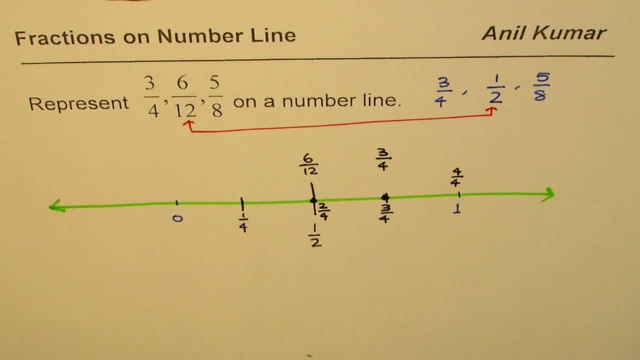 is 3 out of 4. now the question is how to represent 5 out of 8. now one way is you can divide this one into 8 equal parts. that means these are 4 equal parts, one fourth half of those. so so those are. 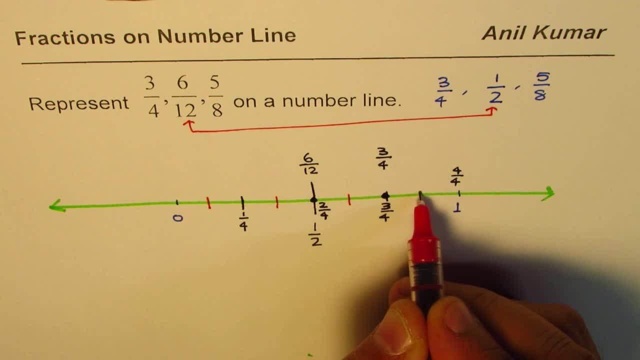 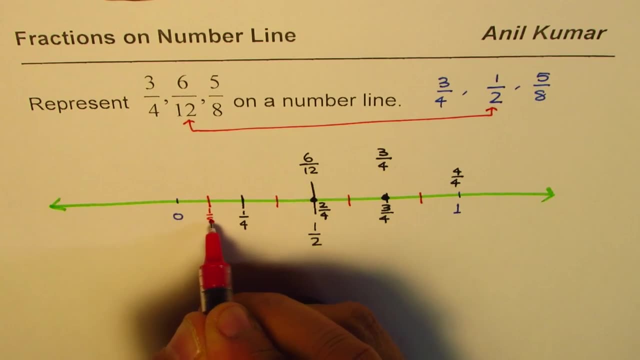 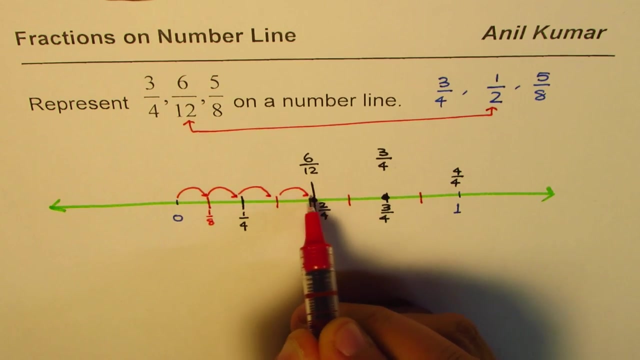 8s: half of this, half of this, half of this and half of this, and then you can count 5. so these are one eighths, right, these are your one eighths. now count 5 of these, and then you can count 4 of them. so this is 1, 2, 3, 4 and this is 5, is it okay? so this one here is 5 out of 8, slightly more. 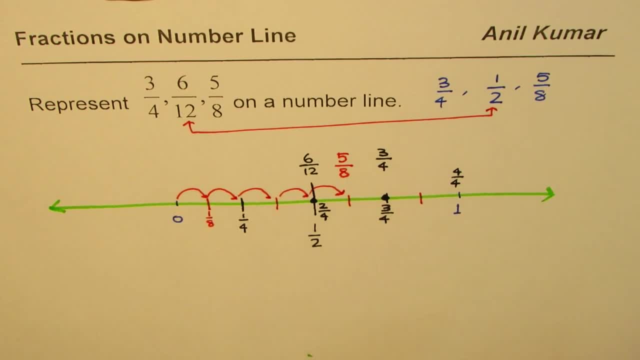 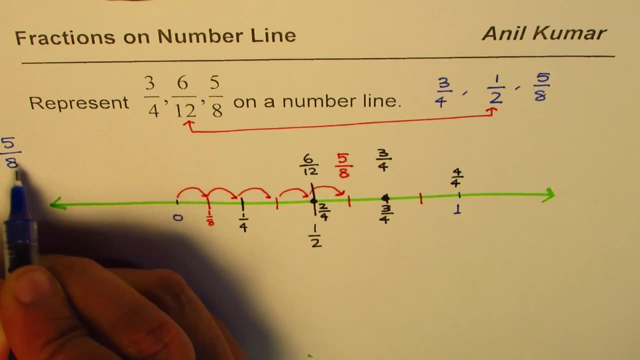 than half correct. you can check if it is right how to check it. that is what we should also do. 5 out of 8- right. think like this: 5 out of 8 is equals to 4 plus 1 out of 8, is that okay? 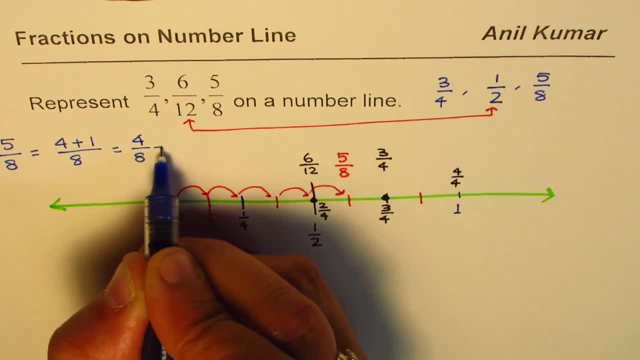 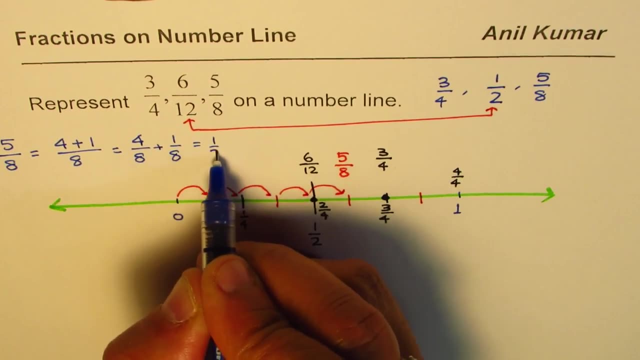 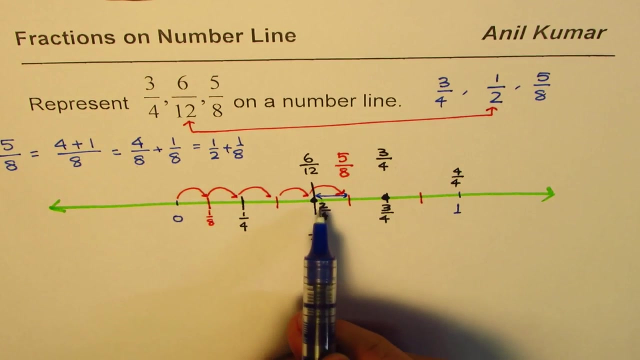 that is 4 out of 8 plus 1 out of 8, 1 eighth more than 4 out of 8. and what is 4 out of 8? it is kind of half right, so half plus 1 eighth. so you'll see this is 1 eighth more than half. do you see that? 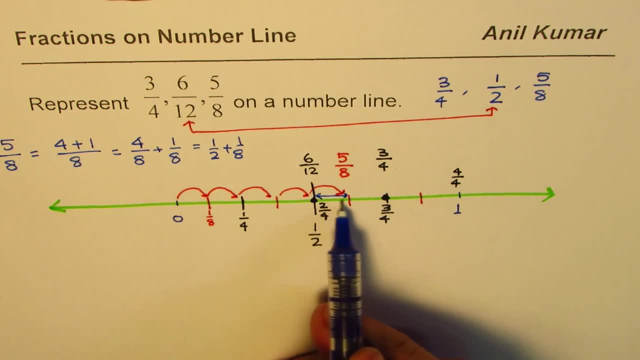 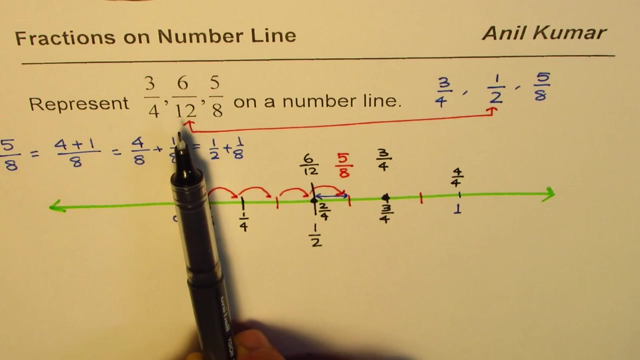 1 eighth more than half, so we could have done like this straight from half also. right, anyway, you've understood how to actually plot the points on a number line when we have different denominators. the idea is to divide the line into the number of pieces- equal pieces, as the denominator is. but more important is, sometimes we may have to simplify. 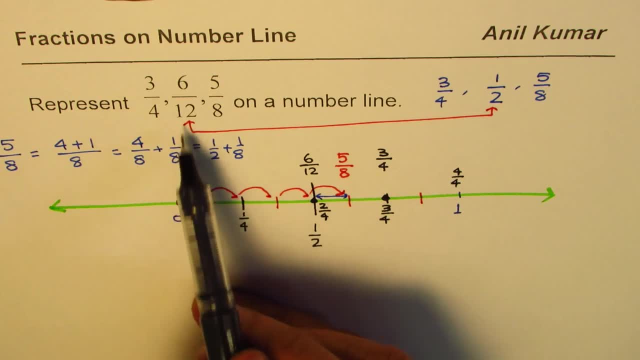 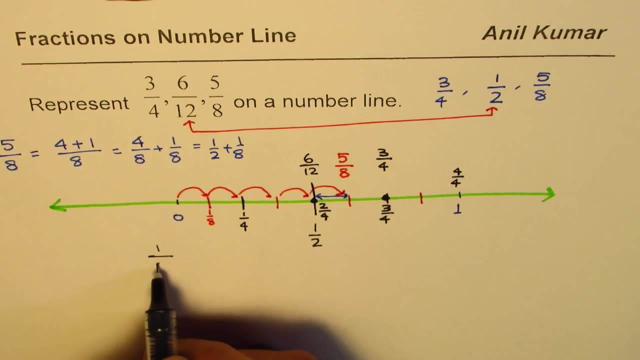 right. so simplify a fraction as we did for 6 out of 12, correct now, based on this, here is the practice question for you. this time i'll give you, like one third right, or we could have some thing over six, five over six, so you can divide into three portions, six portions, and i'll represent. 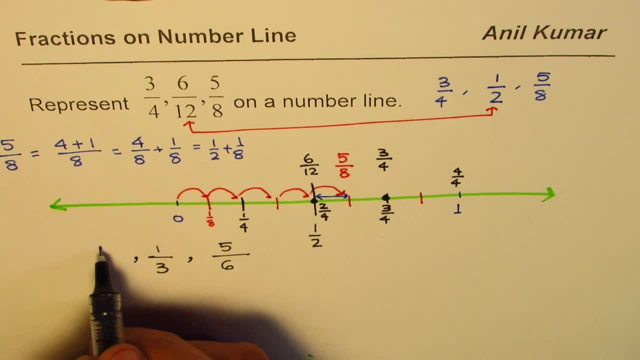 half, in a similar way as i did here. so i'll write four out of eight, right? so sometimes if you start dividing the line to eight equal parts and then go for four, it takes longer. but if you reduce this to half and then do it, it may be a bit shorter time for you, right? so i hope you have understood. 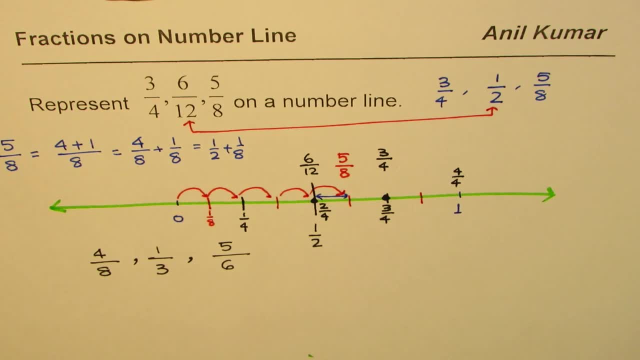 the concept that is for you to practice. so now you can sketch another line and divide this. here is a quick solution. so you'll do like this: you'll draw a line, as we did earlier, mark your zero, okay, and then mark your one. these numbers are between zero and one. i could have given you numbers greater than one also, and then 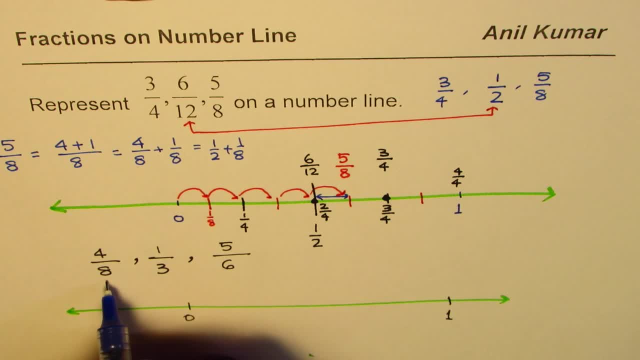 also look at the numbers. four out of eight is same as half, right. so we are actually looking for half, one over three and five over six. so half is easy. go midway and that is your half right. this is your half. so you get your first point, which is half one. third really means that you're dividing into three. 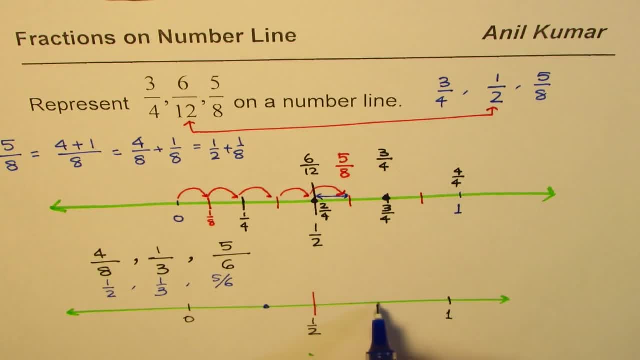 equal parts, right? so let's say these are my three equal parts, right? so these seems to be three equal parts. one third means first right, first one third. one third. five over six means you have to divide these one thirds into their halves. okay, so then you get. then you get one sixth. so each is one. 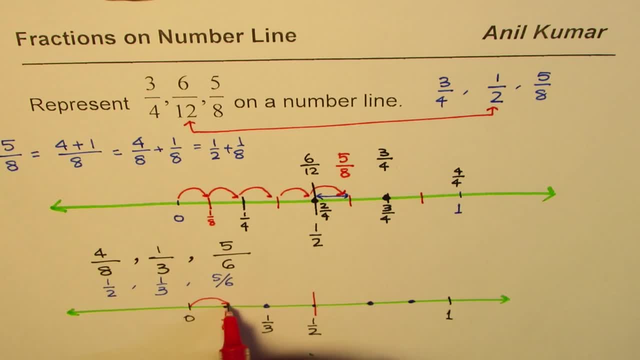 sixth. we are looking for five sixth. that means one, two, three, four and five. five six will be right here. one sixth less than one, so this left out portion will be one sixth. do you see? so that is how you could do it. i hope the concept is clear. thank you and all the best. 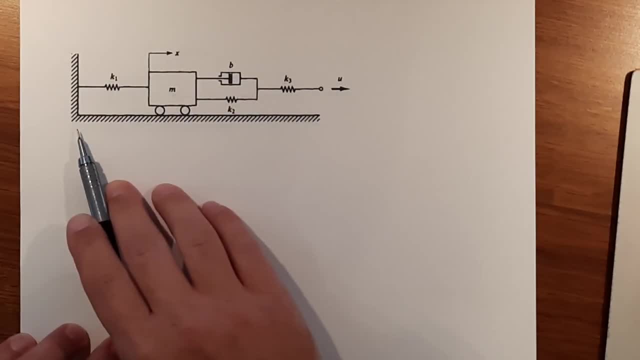 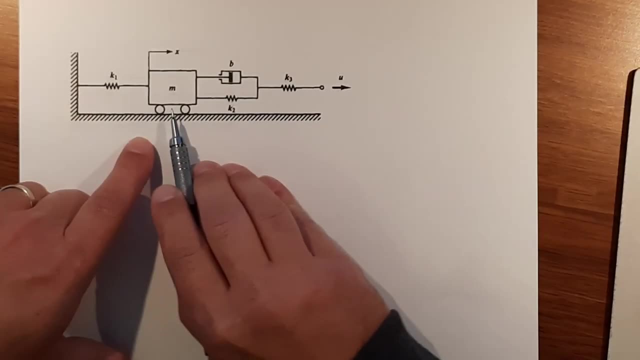 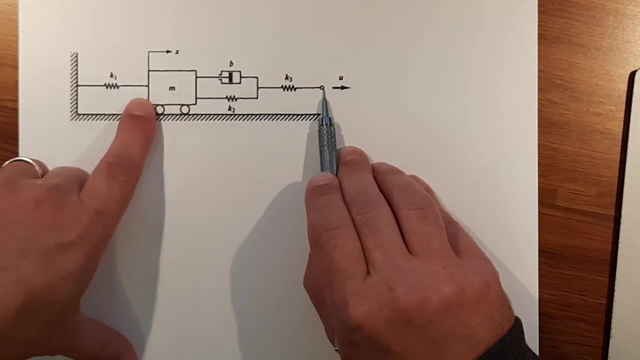 Alright. so today we're going to be writing a mathematical model for this dynamic system. So, to get started, we have a force U that is being applied to this end and we have our output of X. So we're looking at how force U affects the.